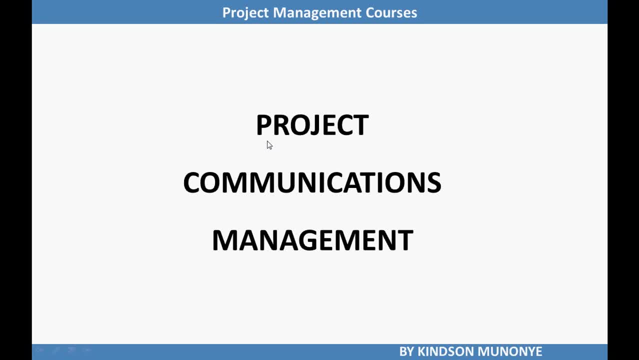 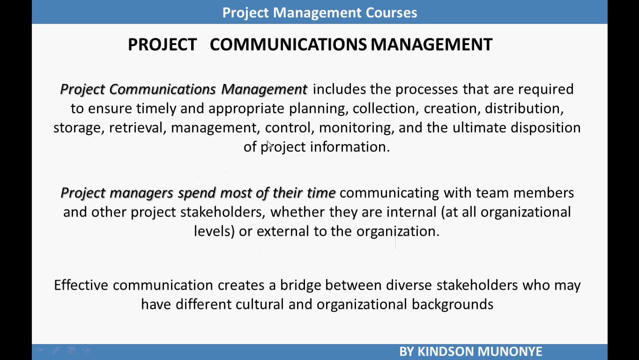 And today we are going to be looking at the three processes in project communications management knowledge area, namely, planned communications management, managed communications and controlled communications. What is project communications management? Project communications management includes the processes that are required to ensure timely and appropriate planning, collection, creation. 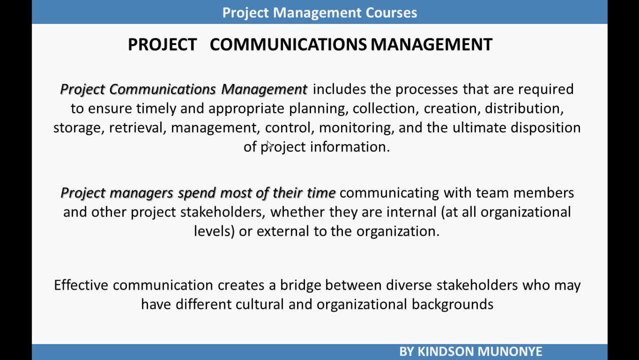 distribution, storage, retrieval, management, control, monitoring and ultimate disposition of information or project's information And project managers spend most of their time communicating with team members and other project stakeholders, whether they are internal or external to the organization. In fact, effective communication builds this. 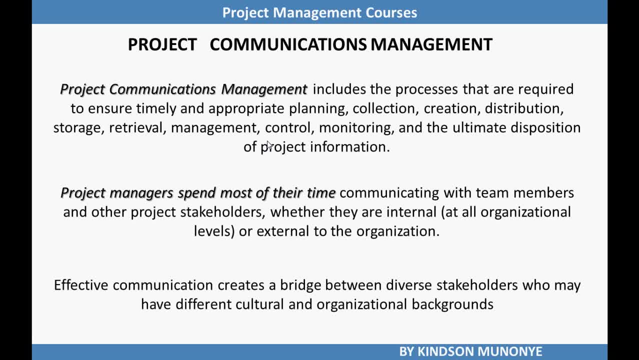 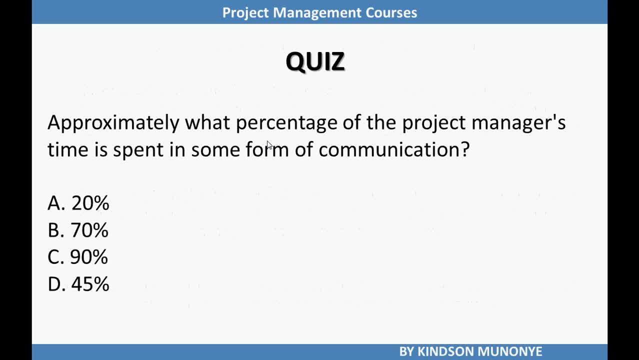 Things like communication management requires a bridge between diverse stakeholders who may have different cultural and organizational backgrounds. Communication management is very important. In fact, one of the key attributes a project manager should possess is communication skills. Let me just give you this important quiz. 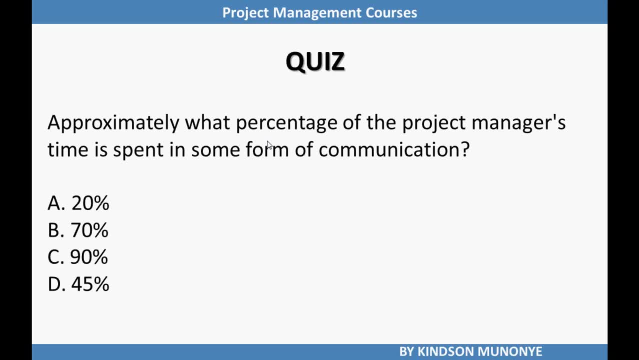 It says approximately what percentage of the project manager's time is spent in some form of communication: 20%, B, 70%, C, 90% and D, 45%. what do you think does it see? 90% project managers spend, or should spend, 90% of their time communicating. all right, let's now look. 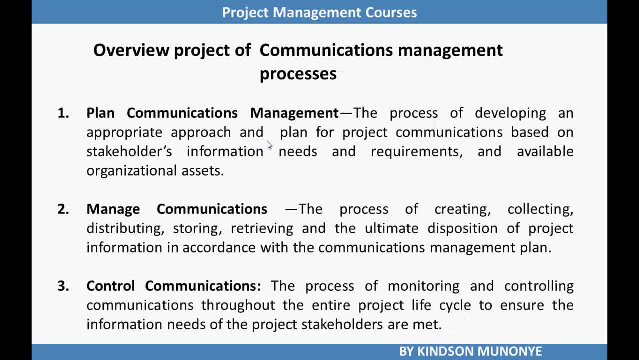 at the processes under the communications management. there are three of them on. the first one is planned communications management, the one we are going to discuss in this very presentation, and that is the process of developing an appropriate approach and plan for project communications based on stakeholders, information, needs and requirements and available. 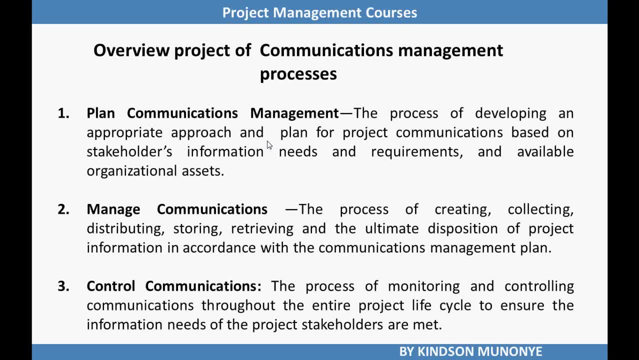 organizational assets. manage communications: the process of creating, collecting, distributing, storing, retrieving and ultimate disposition of project information in accordance with the communications management management plan. control communications: the process of monitoring and controlling communications throughout the entire project lifecycle to ensure the information needs of the project stakeholders are makes. 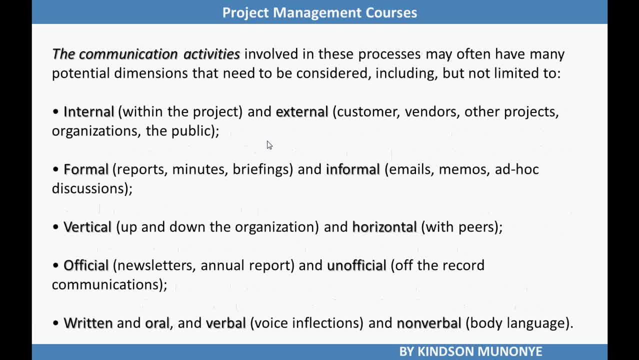 all right. the communication activities involved in these processes may often be, may often have many potential dimensions that need to be considered, including internal within the project output, but not for the internal. the order of participants spends from 不要 standards for those and other project organizations of the public, so we have 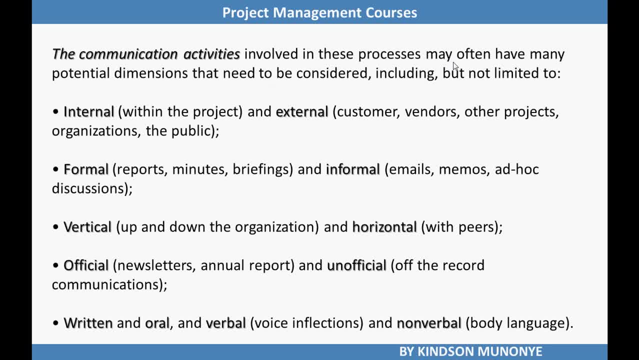 internal and external communication, formerly from our formal means for the applies, report and briefings and minutes of meetings, informal through emails, memos, ad hoc discussions. then we'll have vertical and horizontal web, ander d같ic. we need a algebraic public image, visual damaged, et cetera, as well as гром APB position. we advocate planning and we are very important that we provide information in range of general information. affects the disabilities of officially banning the�istantićit short to them in order to bemi Allah e ethical information or mistake of course, academic safetyometer, discussion services, etc. Compar krieg tag of skills available within national and international, and as well as professionals. 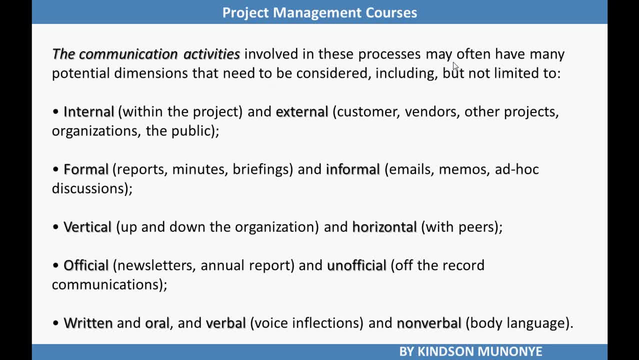 and horizontal. vertical, up and down the organization may high hierarchy in the organizational chart to a lower one and vice versa. and horizontal among PS, let's say among project managers or among project team members in the same level. official and unofficial. when we talk of official, you think of something like newsletters that are circulated, annual reports. unofficial: 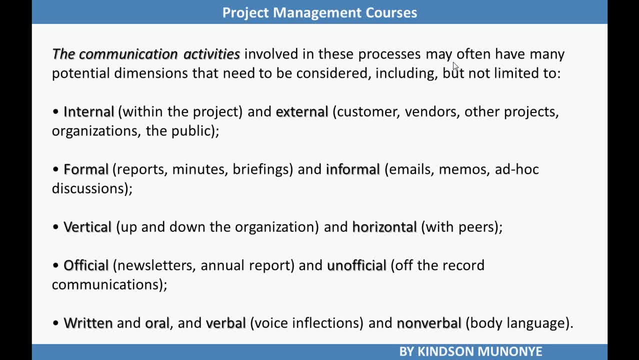 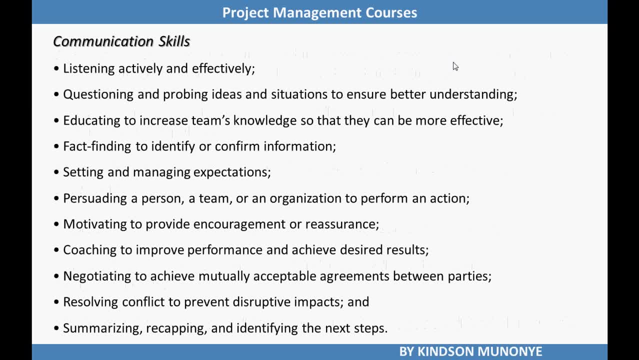 off-the-record communication. then we have written and oral, verbal and non verbal. all right, let's now look at a few communication skills that project managers should possess. one of them is actively listening and also effectively listening, questioning and probing ideas and situations to ensure better understanding. educating to increase teams knowledge so that they can be more. 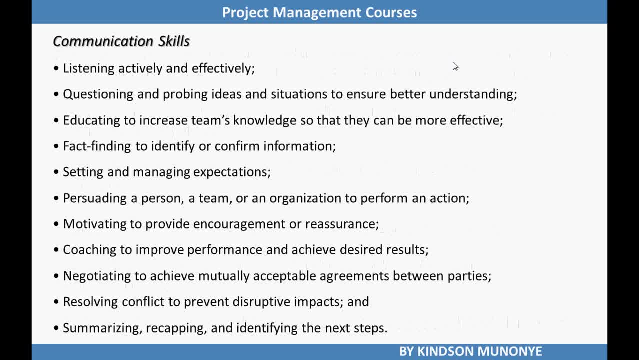 effective and effective at communicating with the team members. effective fact-finding to identify or confirm information. citing and managing expectations. persuading a person, a team or an organization to perform an action. motivating to provide encouragement or reassurance. coaching to improve performance and achieve desired result. negotiating: we discuss negotiation when. 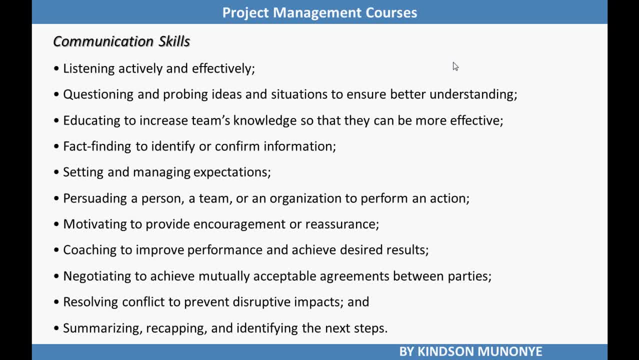 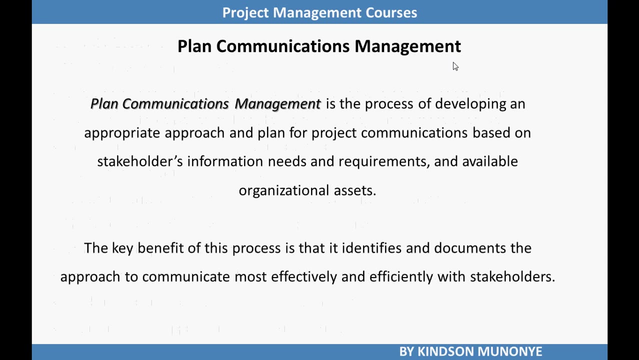 we discuss the tools and techniques use of fire project team. so you need to negotiate, either with functional managers or with other parties, complete resolution methods. we discuss this and manage our project team. they also have a summarizing, recapping and identifying the next steps. these are various communication skills the project manager should possess. so let's now go to 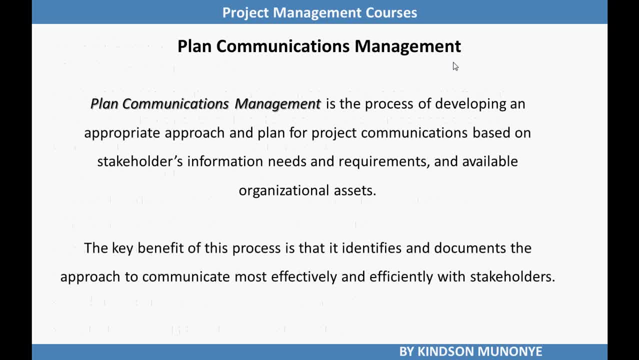 the first knowledge, the first process in the knowledge area, and that is planned communications management. planned communications management is a process of developing an appropriate approach and plan for project communications based on stakeholders, information, needs, requirements and a valuable organizational assets. the key benefit of the planned communication management is that it identifies and 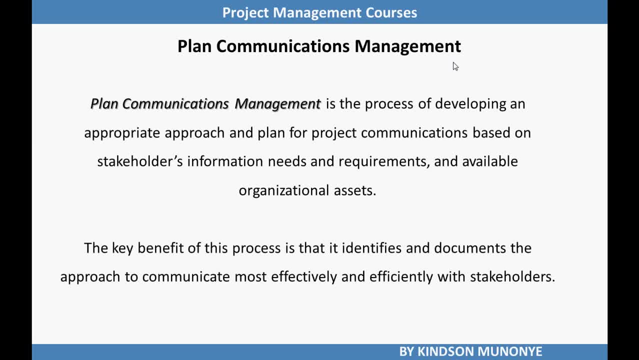 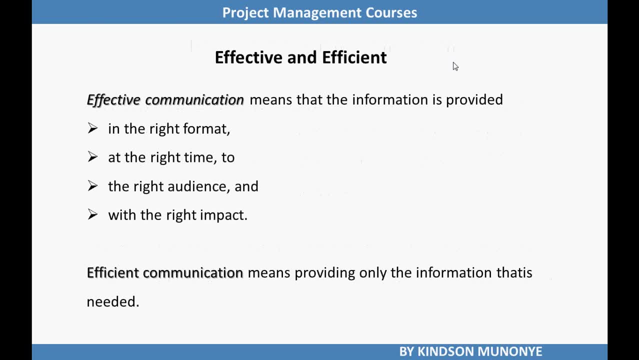 documents, the approach to communicate most effectively and efficiently with stakeholders. now, there are two times I need to be able to differentiate. one is efficient communication. when we have effective communication, effective communication is always highlighted as very important and it means that the information provided should be: one in the right format, two at the right time, three to the right. 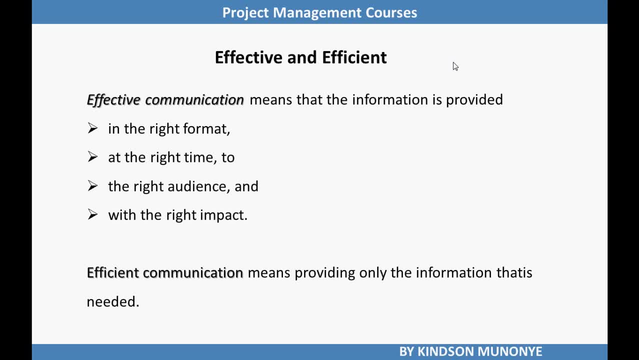 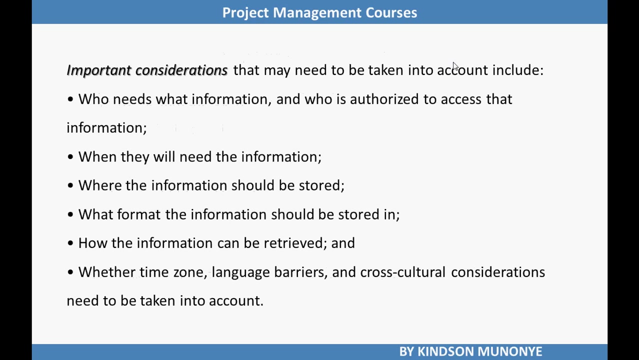 audience. and four with the right impact. if a communication or information meets these four criteria, then we can describe it as effective communication. we also have. efficient communication means providing only the information that is needed. let's also look at important considerations that may be needs that may have to be taken into consideration. for instance, who needs what information and 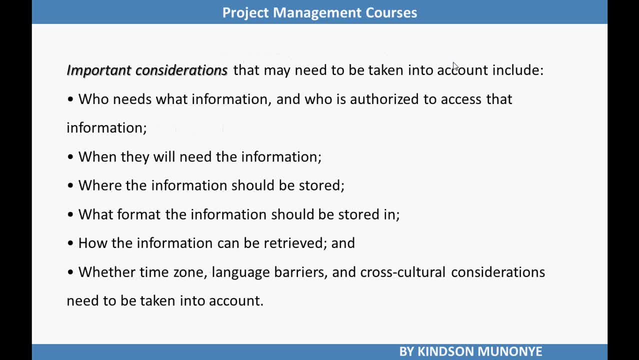 who is authorized to access that information when that is, at the right time where they will need this information, where the information should be stored. we also have what format of the information should be stored in, how the information can be retrieved and whether time zone language barriers across cultural considerations. 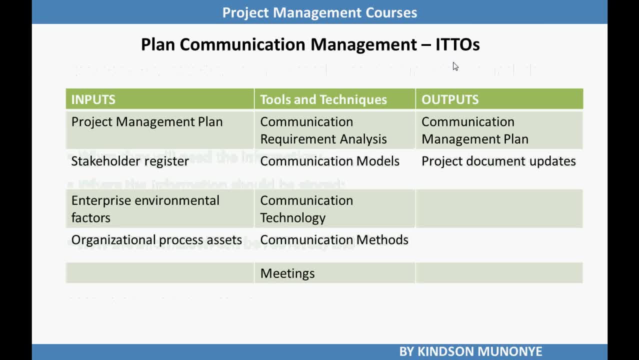 need to be taken into account all right now on to the ITTO's of plan communications management: first, impute this project management plan stakeholder register, enterprise, environmental factors and organizational process assets. the tools and techniques for planned communication include communication requirement analysis, communication models, communication technology. 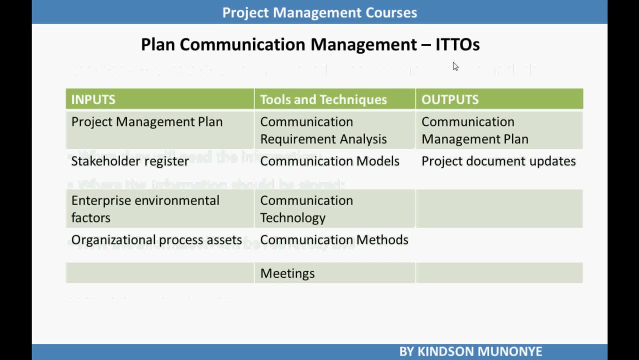 communication methods and readings, the output out to communication management plan and project documents updates. let's now drill down to see why this imputes tools and techniques and outputs are necessary. of course, you know that the project management plan provides information on how the project will be. 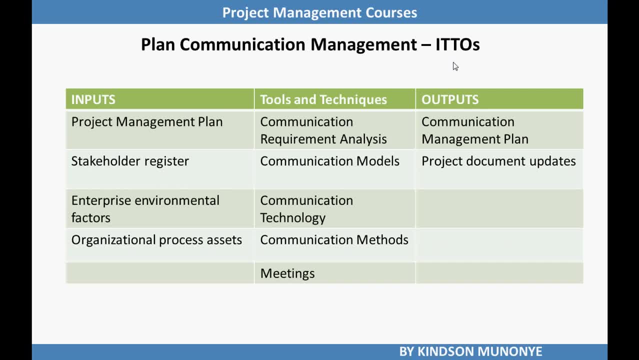 executed, monitored and controlled, as well as closed. so we have project management plan as a necessary impute to plan communications management. the next item is the stakeholder register. it provides the information needed to plan the communication with the project stakeholders. of course, if you are communicating, you are passing information from yourself to someone. 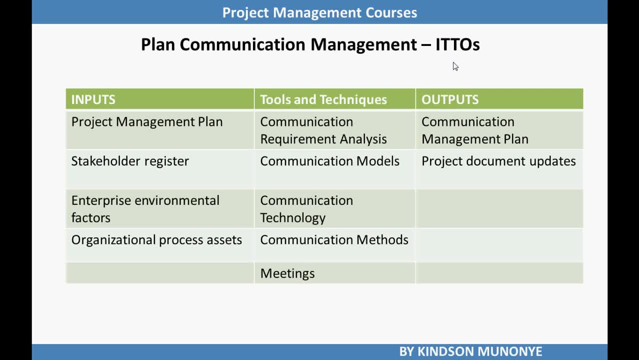 and actually getting information from them. so who are these persons? they are likely documented in the stakeholder register and, of course, we have some enterprise, environmental factors that may affect the communications planning. also organizational process assets. alright, let's now take a closer look at the tools and techniques. 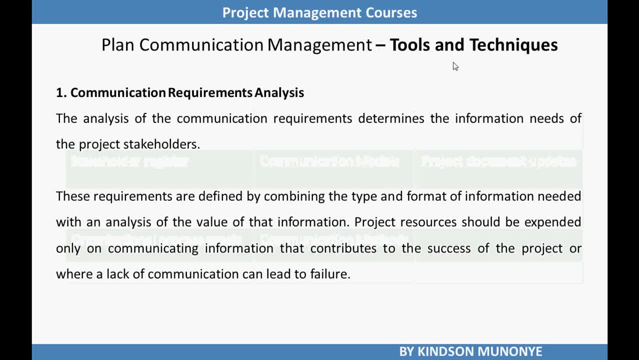 the first one is communications requirements analysis. what is this all about? this is the analysis of the communications requirement and this determines the information needs of the project stakeholders. ok, so we are saying that communication analysis helps you determine the information needs of the stakeholders, these requirements. 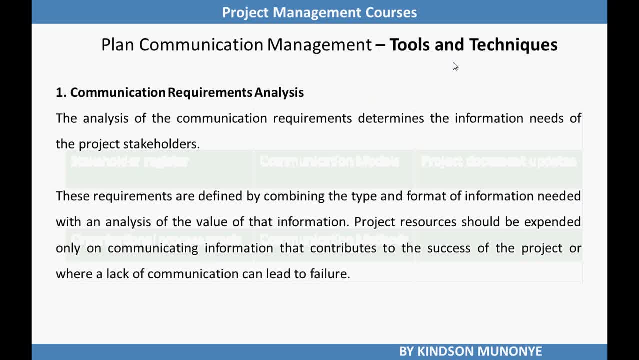 are defined by combining the type and formats of information needed with an analysis of the value of that information. project resource should be expanded only on communicating information that contributes to the success of the project or where a lack of communication can lead to failure. let's continue on communication requirements analysis. 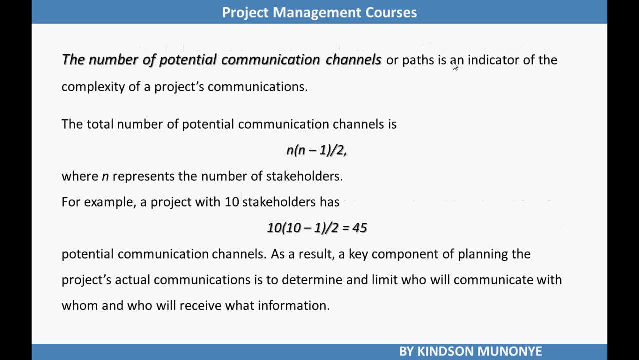 there is a little more information in the questionnaire content. the functionality of communications requirements analysis is 경 elemento. a little mathematics there, but never mind, it's not difficult. the number of potential communications channel on the communication requirement analysis, the number of channels or paths is an indicator of the complexity of the 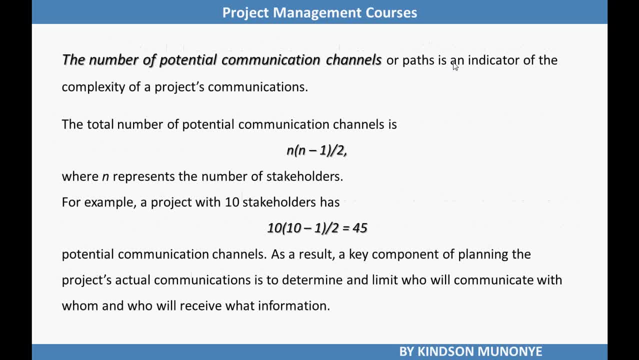 project communication. so the total number of potential communication channel is given by this formula: n into n minus 1 over 2. so let's assume okay, where n represents the number of stakeholders. so let's take for instance three stakeholders: one, two, three. so number of communication pathways is 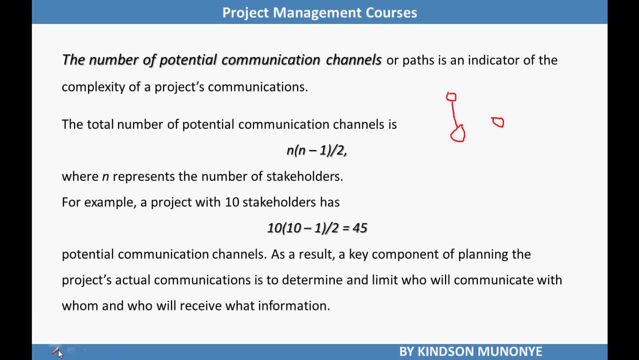 just a minute, let me change the color of this channel. all right, let me, let me use a different color to do this. so okay, let's use green. so now a 1, 2, 3. so how many channels you see? one, two, three. so then you see the channel of communication goals. 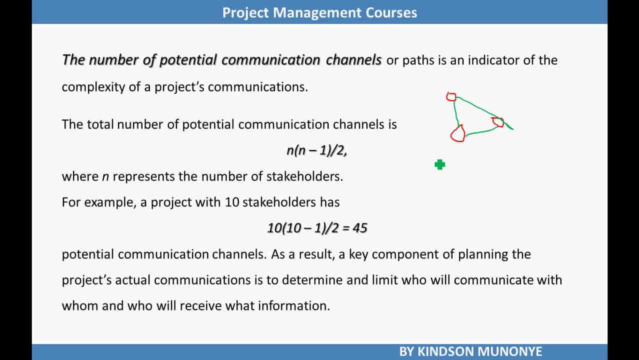 so stop shown here. before anything else, let's get back to the next part of the solution. um, you can take 2 channelften. better way, is there? um, what is the something about channel math? so smile, okay. so now how to put the key? we don't. 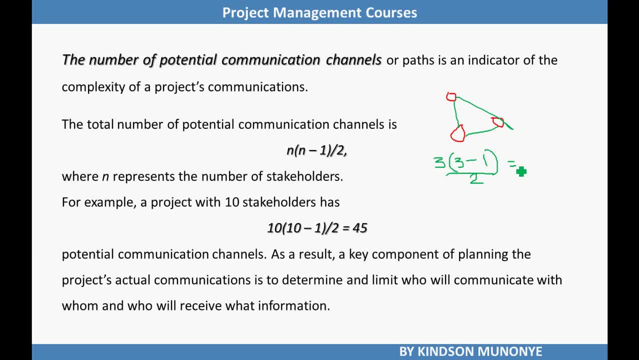 give us any question. okay, if order is n and n plus n minus n, and we do that, the second part of the game, uh, we are going to start with. so n plus n changes the times. 3 minus 1 is 2 over. what Over 2? and that gives us what Equals 6 over 2. 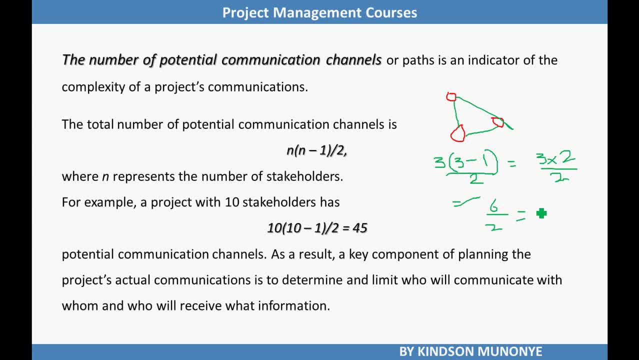 equals what Equals 3? okay, so meaning that there are three stakeholders, we have three again. let me just do a different test and let's see if it works. let's assume four, one, two, three, four, let's say four stakeholders, how many communication channel are we going to have? now we are going to draw the paths. 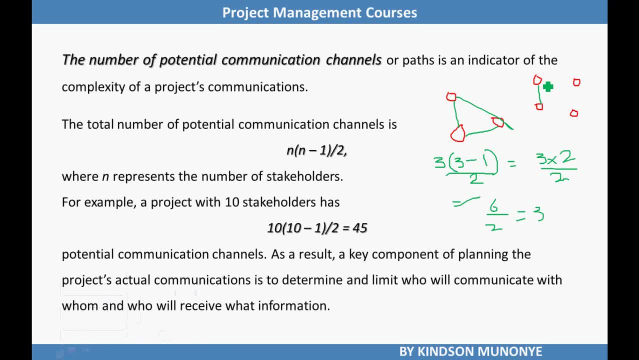 and then we do the same thing again. let's do the calculation: one, two, three, four, five, six. so what we are saying is that if we have four stakeholders, then we need how many channels? we of course need six channel. so if you are going to calculate it, we have four into. 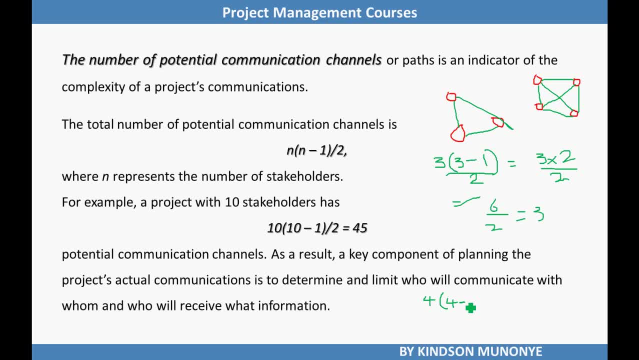 four minus one over two. so if you do the maths, you see that it's going to give us four times three over two, twelve over two, six. that justifies what we have here. so you need to memorize this formula. that is part of communications requirements analysis: a calculation of the number of channels for a. 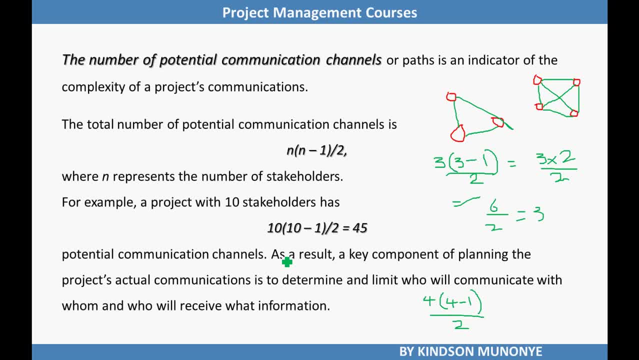 given number of stakeholders. so, as a result, key component of planning the project's actual communication is to determine and limit who will communicate with whom and who will receive the information. so that planning is necessary, because the more the number of stakeholders to pass information, the more complex the number of the communication is going to be. so it's. 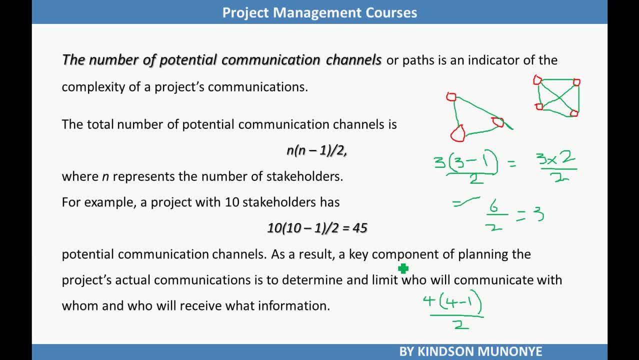 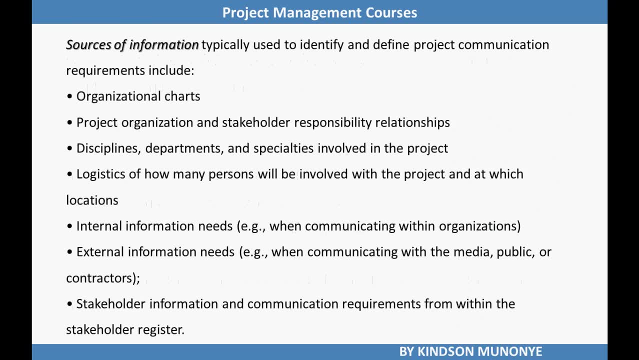 better to simplify by reducing the number of channels for a given number of stakeholders. the number of channels- and this we do by deciding who and who deserves the information. also of importance is a sources of information typically used to identify and define project communication requirement, and they include organizational chats, projects, organization. 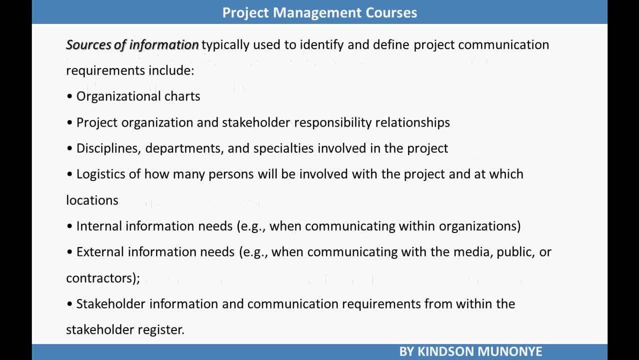 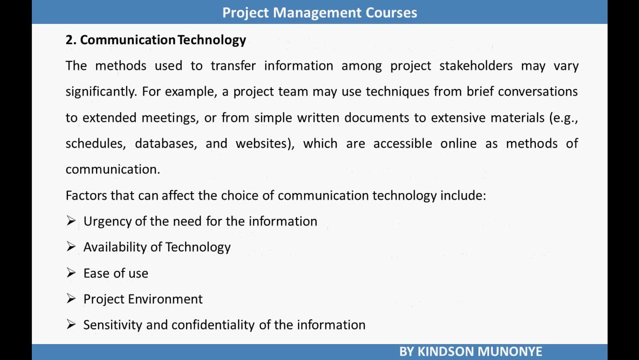 and stakeholder: responsibility relationships, disciplines, departments and specialties involved in the project, logistics of how many persons will be involved with the projects and at which locations. internal information needs. external information, needs of stakeholder information and communications requirement from within the stakeholder register. these are the sources of information. the next tool and 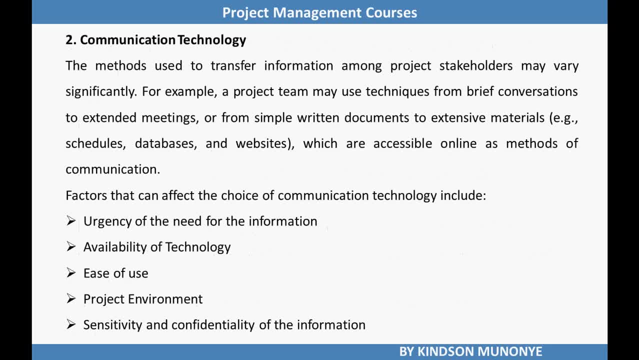 technique of importance in planned communication management is the communication technology. communication technology follows the communications requirements analysis and communication technology for short. you know ICT is always a very important in every organization. the method used to transfer information among project stakeholders may vary significantly. for example, a project team may use techniques. 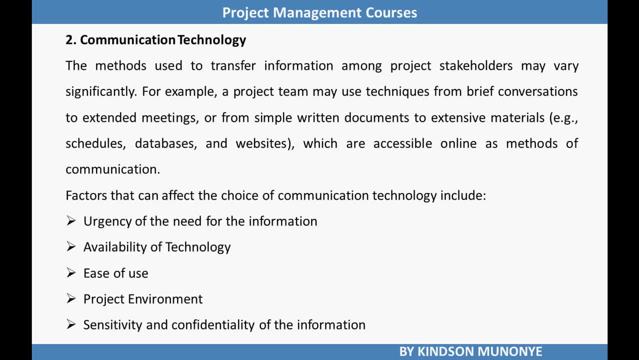 ranging from brief conversation to extended meetings, or from simple written documents to extensive material, or from guided emails to's favorite materials, to customer security. there are a number of factors that can affect the choice of communication technology which are accessible online as methods of communication. factors that can affect the choice of communication technology. 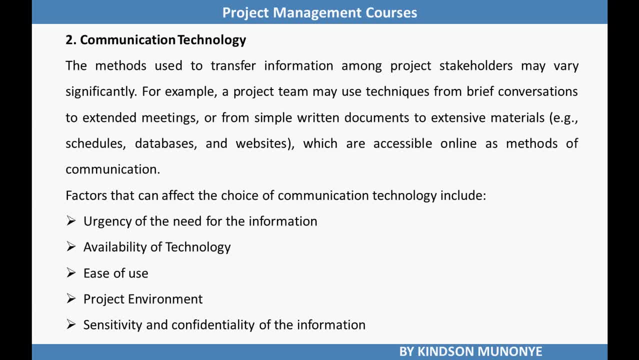 include urgency of the need for the information, availability of technology, ease of use, project environment sensitivity and confidentiality of the information. so this can affect the choice of communication technology to use. will it be a two-way radio? will it be providing communication technology on a regular basis? 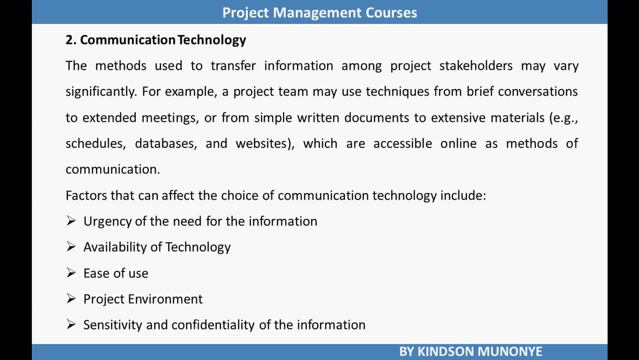 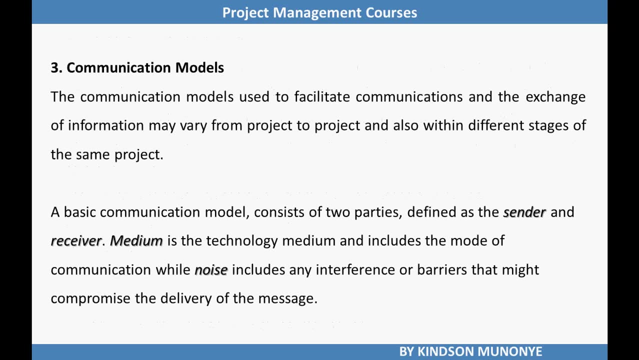 GSM cell phones for users. Will it be providing tablets for communication email facilities? This has to be decided and factors like these listed here needs to be taken into consideration. Another tool and technique used in planned communication management is communication models. Now, communication model is different from communication technology, but also different from 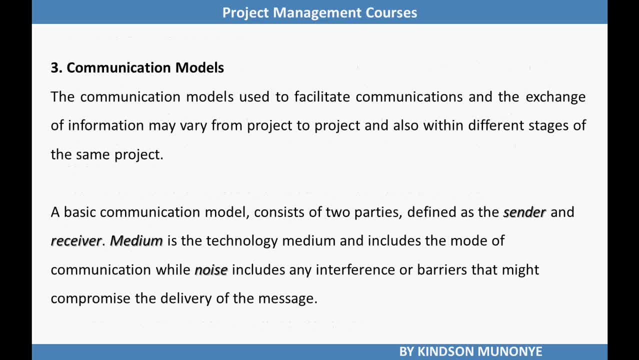 communication methods. Communication model used to facilitate communication and exchange of information vary from project to project. A basic communication model consists of two pathways, defined as the sender and the receiver. Medium is the technology medium that includes the mode of communication, while noise includes any interference or barriers that might compromise. 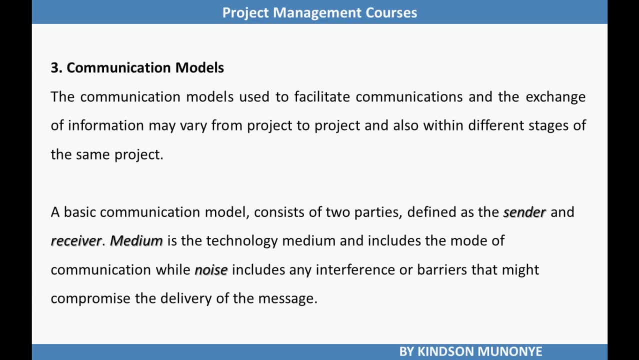 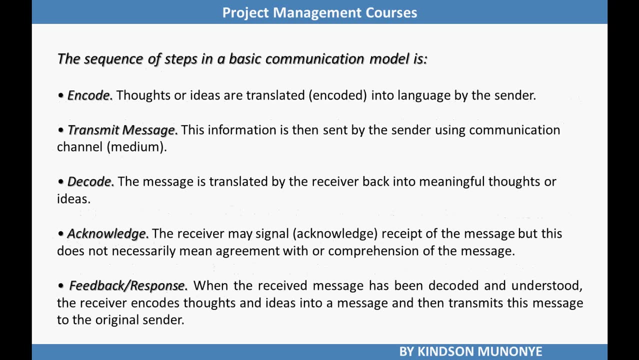 the delivery of the message. So when we talk of communication models, take note of items like components, like sender, receiver, medium and noise. Alright, still on communication model, the sequence of steps in a basic communication model is: the first one is encode. That means that thoughts or ideas are translated, or 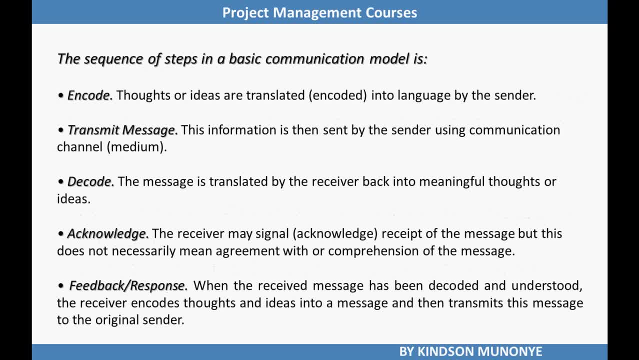 encoded into language by the sender. So it means that the sender or receiver originates the information and before you are going to send it out you need to encode it into a language that can be received by the receiver. Then we have you. now, after encoding, you transmit the message. Information is then. 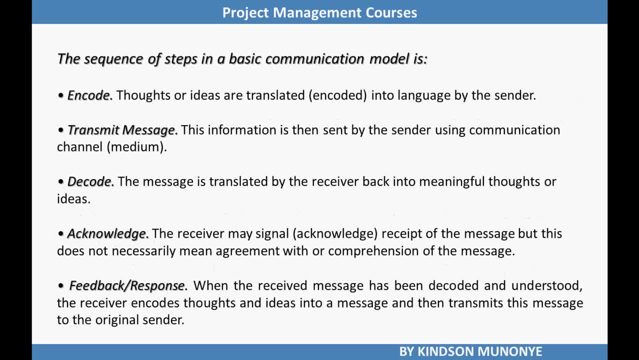 sent by the sender using communication channel. The next is decode. This happens as the receiver sends. the message is translated by the receiver back into meaningful thoughts or ideas, Then at the receiver's end we have acknowledge. The receiver may signal acknowledge received all the info of the message, but this does not necessarily. 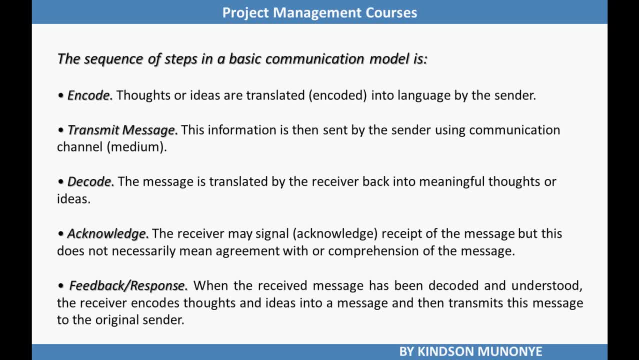 mean agreement with or comprehension of the message. So acknowledgement simply means: oh yes, I received it, I got it. Then the next one, finally, feedback or response, when the receiver message has been decoded and understood. The receiver encodes thoughts and ideas into a message and transmits this message to the 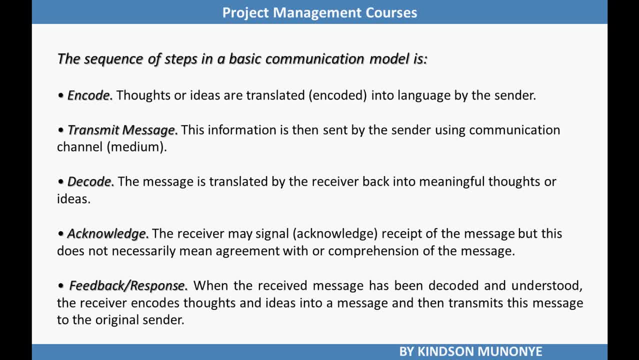 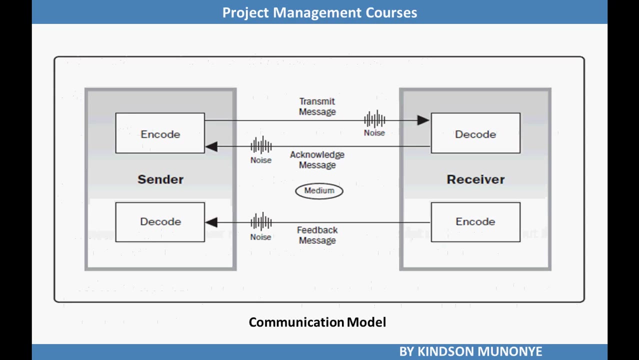 original sender. So this is different from acknowledge. The feedback is a response. You've understood the message and now you are giving a response based on the information contained therein. So these are the steps, or sequence of steps in a communication model. Yes, this picture came from the Pinball Guide 5th edition. that shows us the steps, or 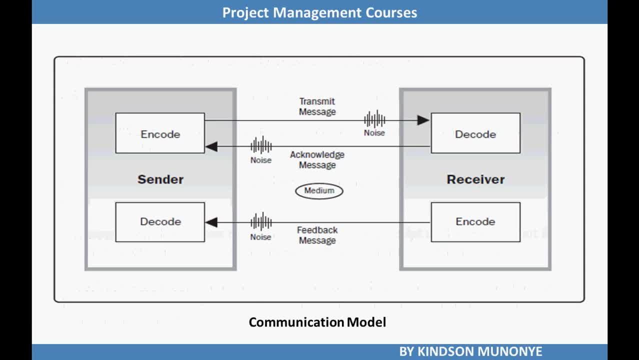 sequence in a communication model. We have encode. okay, transmit message. Let's take it serial, one after the other. This is the sender. this box represents the sender. this box represents the receiver. In between, here is a medium of transmission, or. 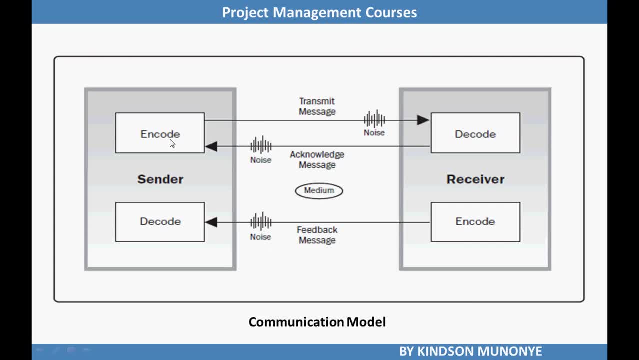 the channel. All right. so the sender encodes okay and transmits message. There might be noise in between. The receiver decodes the message and acknowledges the message. After that the receiver again encodes a feedback message and sends it right back to the sender. So that's about communication models. Let's now 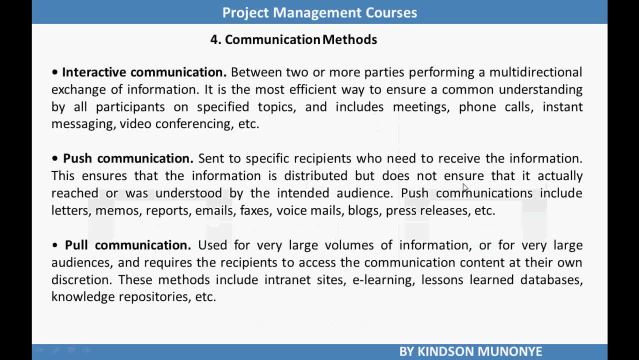 look at communication methods. There are three, three different communication methods described in the Pinball Guide 5th edition. One of them is interactive, push communication and pull communication. Let's look at this. Interactive is between two or more parties performing a multi-directional. 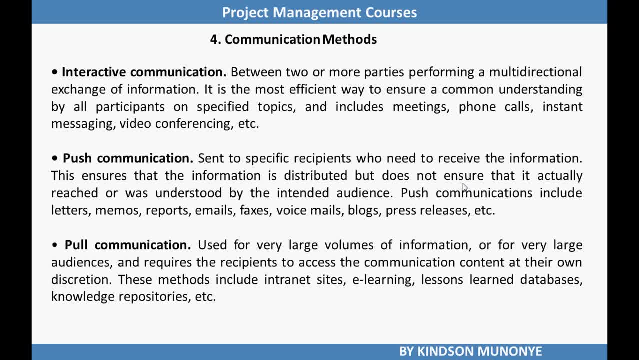 exchange of information. This is the most efficient way to ensure a common understanding by all participants on specified topics. Examples of interactive communication are meetings, phone calls, instant messaging or chats and video conferencing. Then we also have push communication. This message is sent to specific resources like a Facebook group or a Facebook 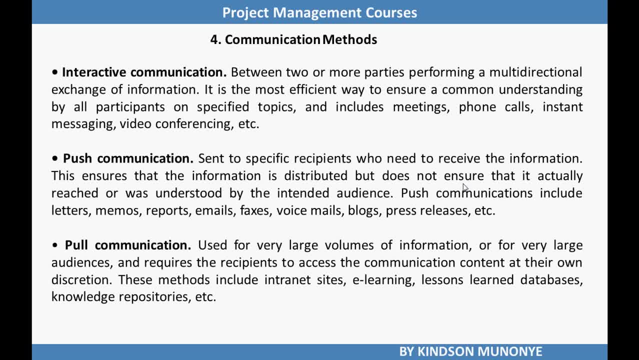 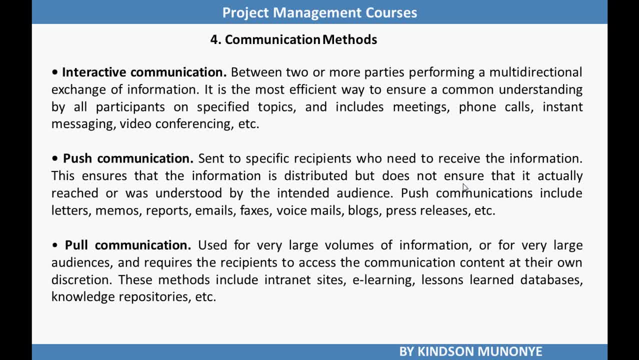 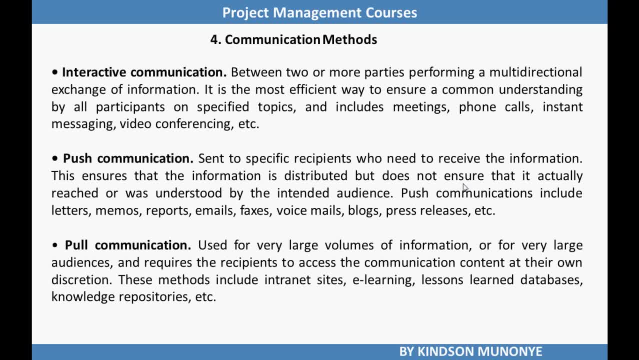 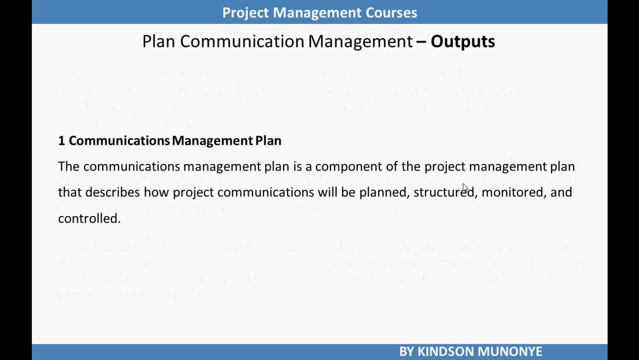 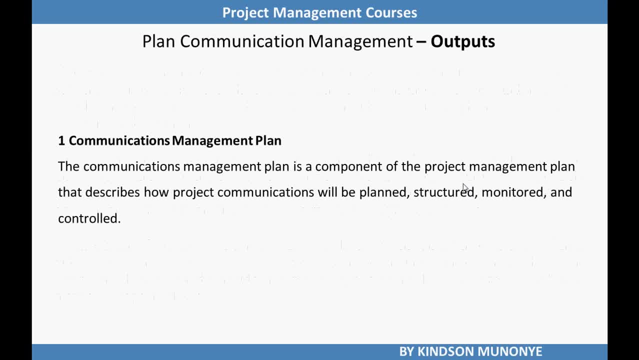 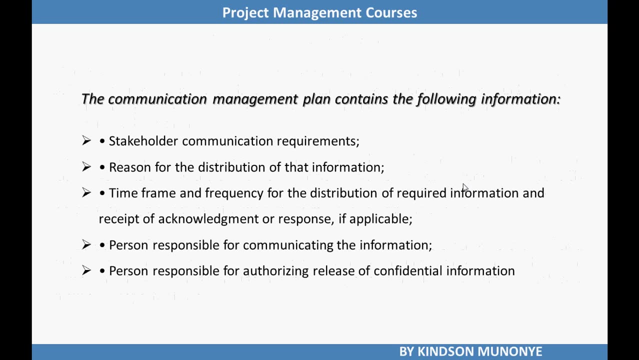 communication management plan is a component of the project management plan that describes how project communication should be planned, structured, monitored and controlled. The communication management plan contains the stakeholder communication requirement, the reason for the distribution of that information, timeframe and frequency for the distribution of required information, and. 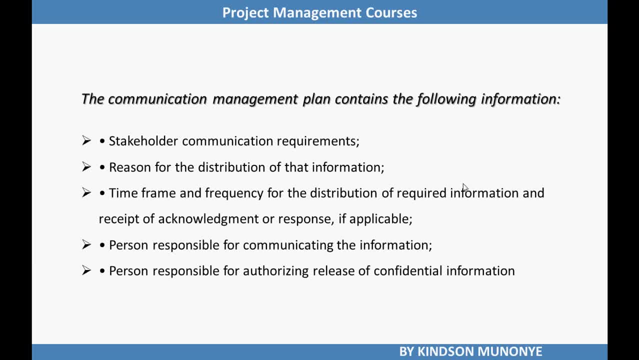 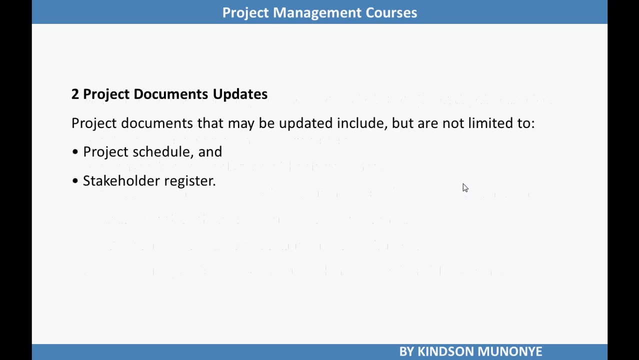 receipt of acknowledgment or response, if applicable, person responsible for communicating the information and person responsible for authorizing the release of confidential information. And then, finally, we have, as an output of planned communication management, the project document updates. the project document updates might be project schedule and stakeholder register.